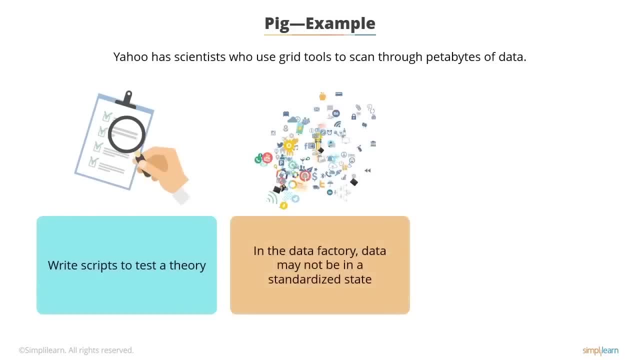 However, in the data factory, data may not be in a standardized state. This makes PIG a good option, as it supports data with partial or unknown schemas and semi- or unstructured data. There are two major components of PIG. 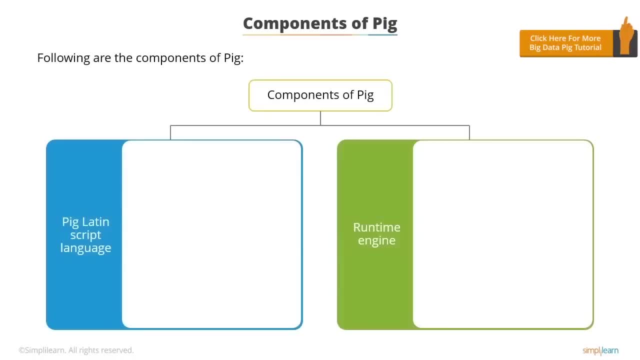 PIG and Data Factory. PIG- Latin script language, A runtime engine. The PIG Latin script is a procedural data flow language. It contains syntax and commands that can be applied to implement business logic. Examples of PIG Latin are: load and store. The runtime engine is a compiler that produces sequences of MapReduce programs. 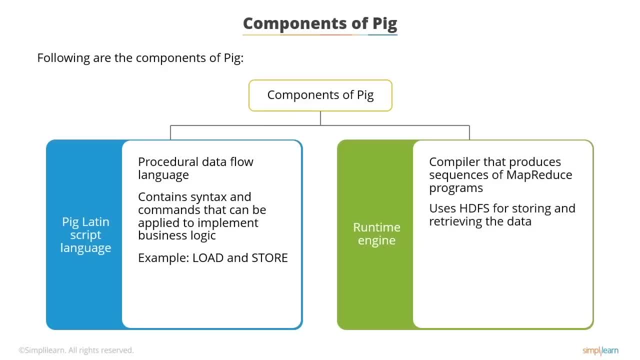 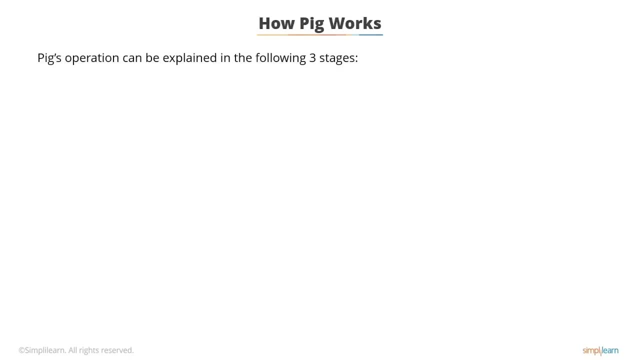 It uses HDFS to store and retrieve data. It is also used to interact with the Hadoop system, HDFS and MapReduce. The runtime engine parses, validates and compiles the script operations into a sequence of MapReduce jobs. PIG's operation can be explained in three stages. 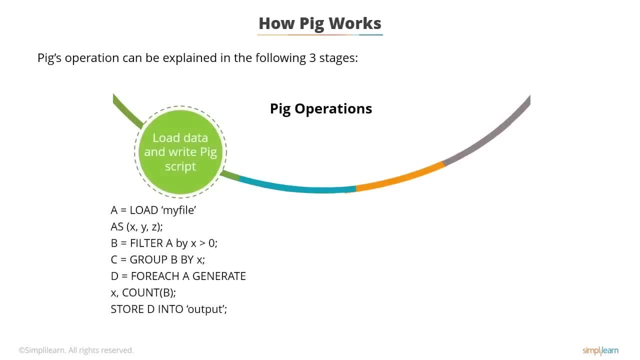 In the first stage, the data is loaded and a PIG script is written. In the second stage, the PIG execution engine parses and checks the script. If it passes, the script is optimized and a logical and physical plan is generated for execution. 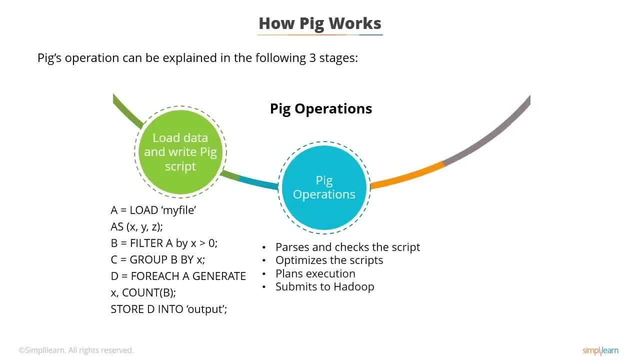 The job is submitted to Hadoop as a job comprising of Map and Reduce tasks. PIG monitors the status of jobs using Hadoop API and reports the status to its client In the execution stage. the results are dumped onto the screen or are stored in HDFS, depending on the user command. 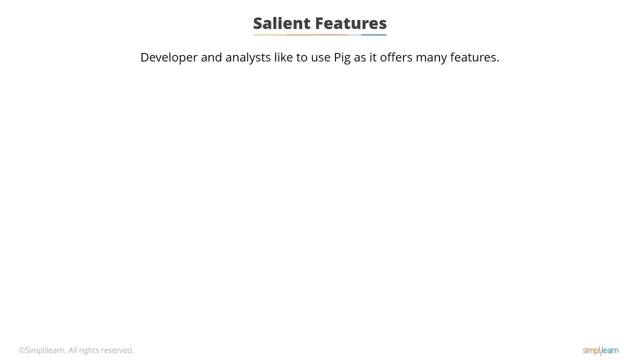 Developer and analysts like to use PIG, as it offers many features. Some of the features are as follows: Provision for step-by-step procedural control and the ability to operate directly over files Schemas that, though optional, can be assigned dynamically. Support to user-defined functions, or UDFs, and to various data types. 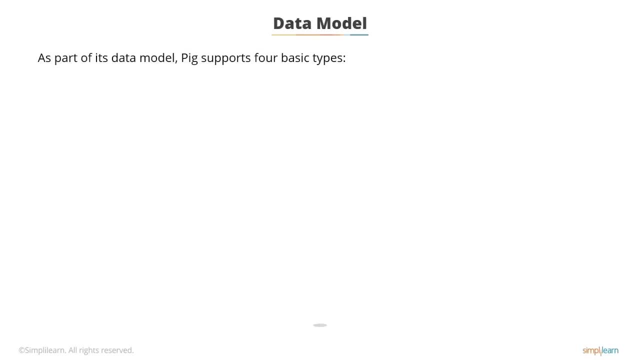 As part of its data model, PIG supports four basic types. The first is Atom, which is a simple atomic value like integer, long, double or string. The second is Tuple, which is a sequence of fields that can be of any data type. 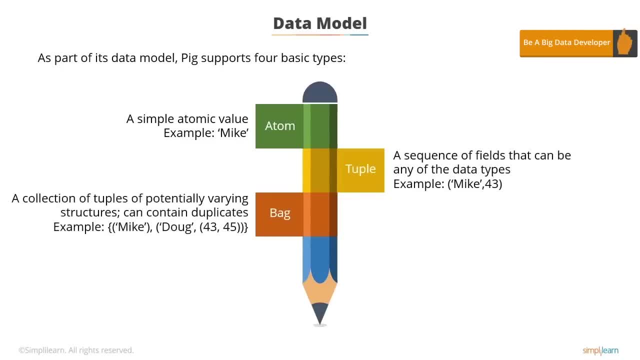 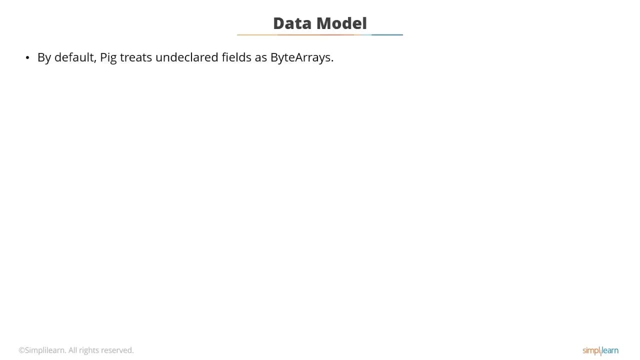 The third is Bag, which is a collection of tuples of potentially varying structures and can contain duplicates. Finally, there is Map, which is an associative array. The key must be a character array, but the value can be of any type. By default, PIG treats undeclared fields as byte arrays, which are collections of uninterpreted bytes. 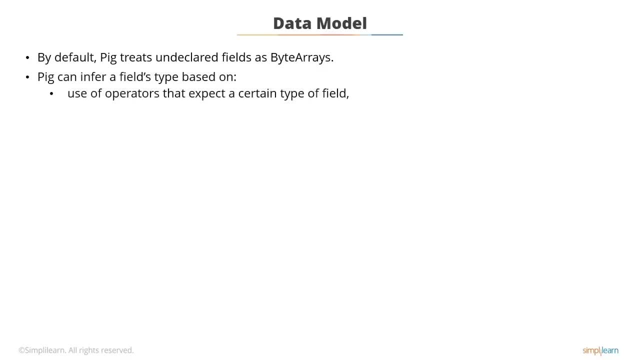 PIG can infer a field's type based on the use of operators that explain a certain type of field. It can also use user-defined functions, or UDFs, with a known or explicitly set return type. Furthermore, it can infer the field type based on schema information provided by a load function. 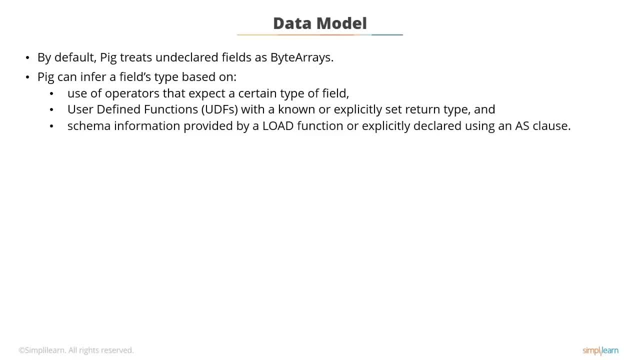 or explicitly declared using an AS clause. Please note that type conversion is lazy, which means the data type is enforced at the point of execution Only. PIG Latin has a fully nestable data model with atomic values, tuples, bags or lists and maps. 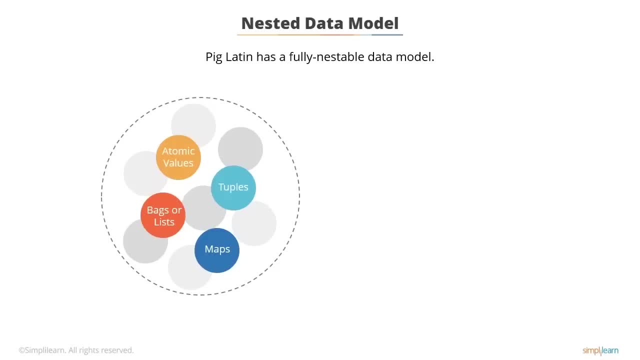 This implies one data type can be nested within another, as shown in the image. The advantage is that this is far more natural to programmers than flat tuples. Also, it avoids expensive joins. PIG works in two execution modes: local and mapper-duce. 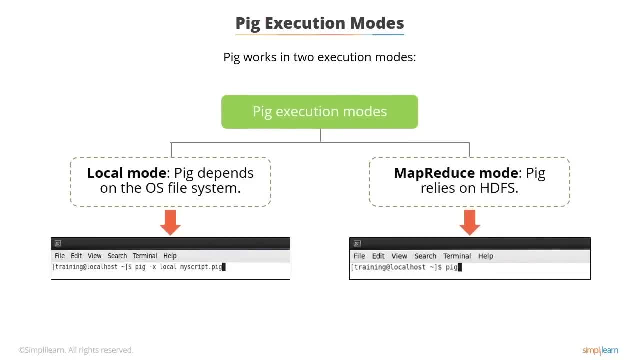 In the local mode. the PIG engine takes input from the limiter, which will stop it from moving to any future model. The randomization of the PIG is done by the disk pointer, but the logic is different: takes input from the Linux file system and the output is stored in the same file system. 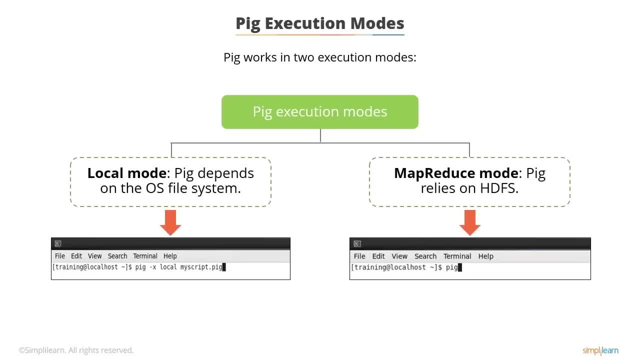 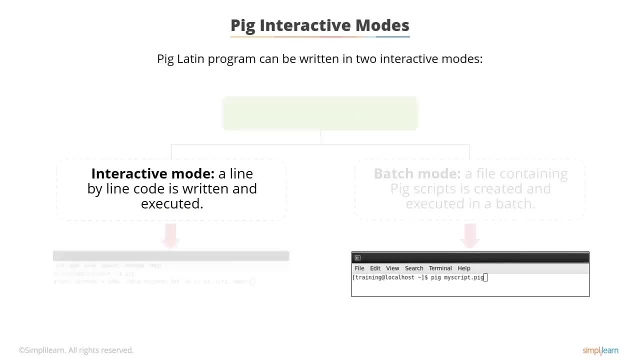 In MapReduce mode the PIG engine directly interacts and executes in HDFS and MapReduce. The two modes in which a PIG Latin program can be written are interactive and batch. Interactive mode means coding and executing the script line by line as shown in the image. In batch mode. 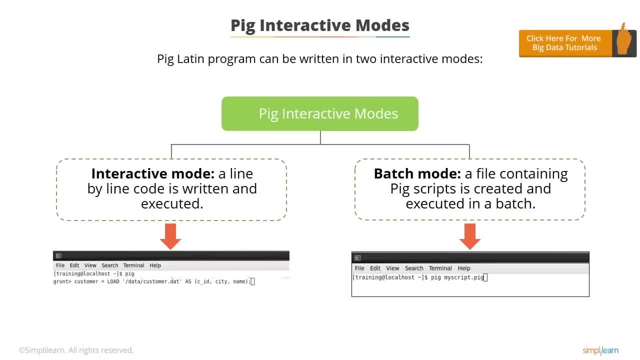 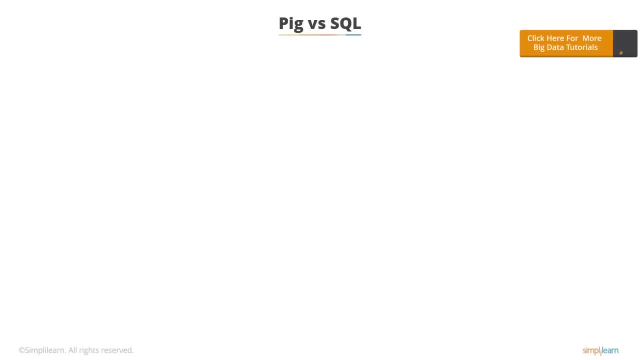 all scripts are coded in a file with the extension pig, and the file is directly executed. Since we have already learned about Hive and Impala, which work on SQL, let's now see how PIG is different from SQL. The first difference between PIG and SQL is: 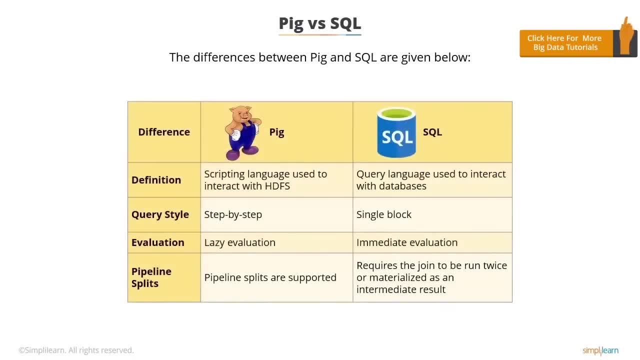 that PIG is a scripting language used to interact with HDFS. SQL is a query language used to interact with databases residing in the database engine. In terms of query style, PIG offers a step-by-step execution style compared to the single-block execution style of SQL. 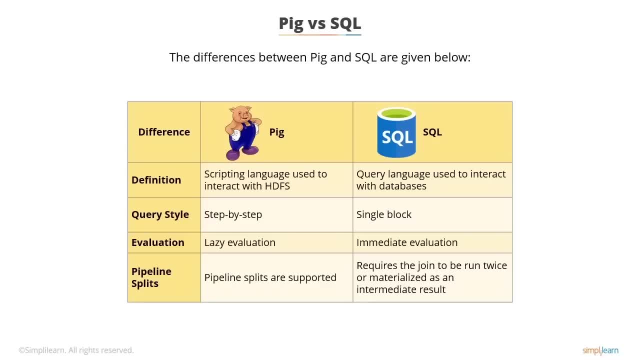 PIG does a lazy evaluation, which means that data is processed only when the store or dump command is encountered. Also, SQL offers immediate evaluation of a query. Pipeline splits are supported in PIG. However, in SQL, you may need to run the join command twice for the result to be. 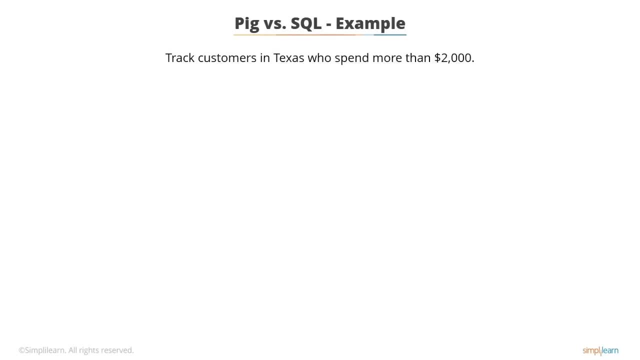 materialized as a query. Now that we've gone through the differences between PIG and SQL, let us now understand further with an example. The illustration given is an example to help you understand the SQL command and its PIG-equivalent command script. 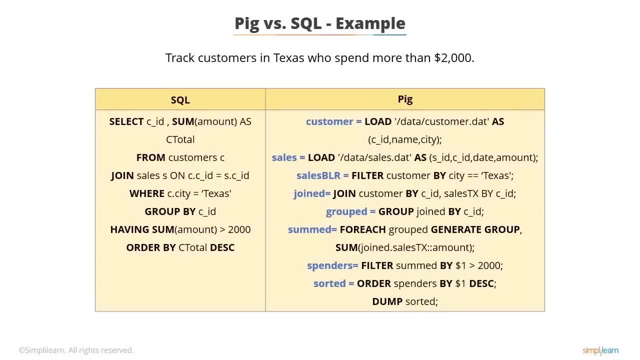 The SQL command focuses on the customer table with columns CID and CTOTAL, which is the sum of the amounts It joins the sales table. with reference to CID, where the C city is Texas, The grouping of CID is performed by ensuring the sum of the amounts. 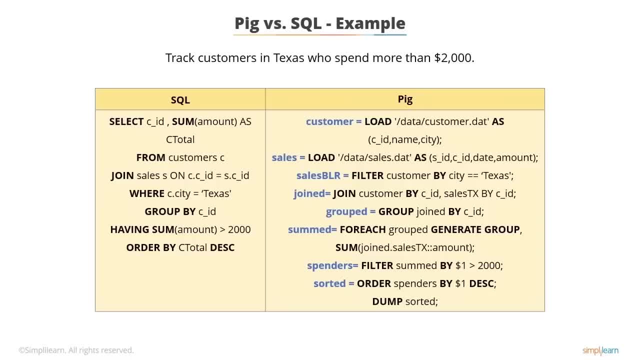 is greater than the 2,000 ordered in descending order. Now examine the same function using PIG. In PIG you create two entities, customer and sales, where you load equivalent data with the schema. You filter the customers based on location, for example, Texas. 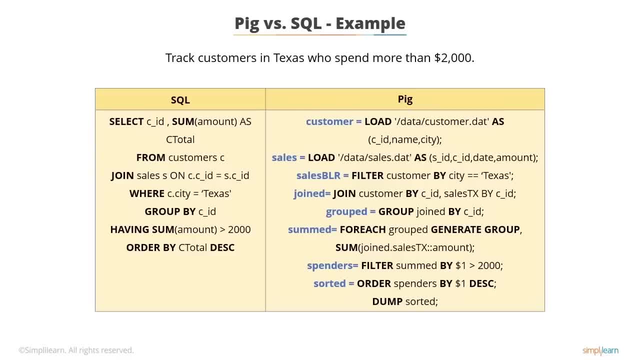 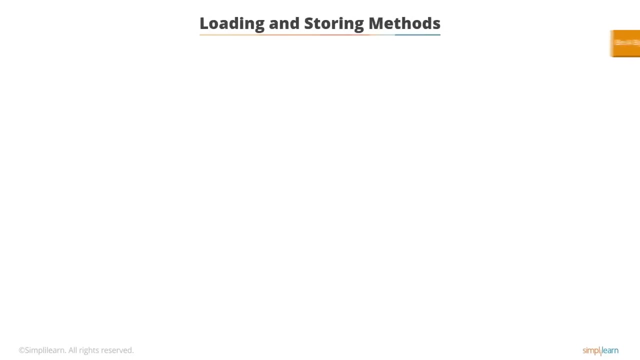 Both data are joined using the CID row. The sum of the amounts of the individual CIDs is calculated. Now isolate those customers who spend more than $2,000.. Later sort the customers in descending order. Now let's look at how to load and store data in the PIG engine using the command console. 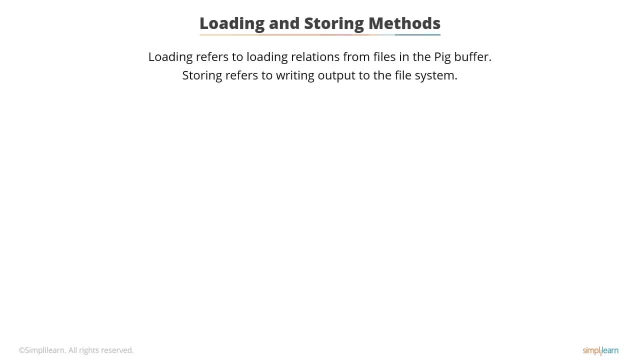 Loading refers to loading relations from the files in the PIG buffer. This is done using the keyword LOAD, followed by the name of the variable for which data is to be loaded. A series of transformation statements processes the data Storing refers to writing output to the file system. This is done using the keyword STORE. 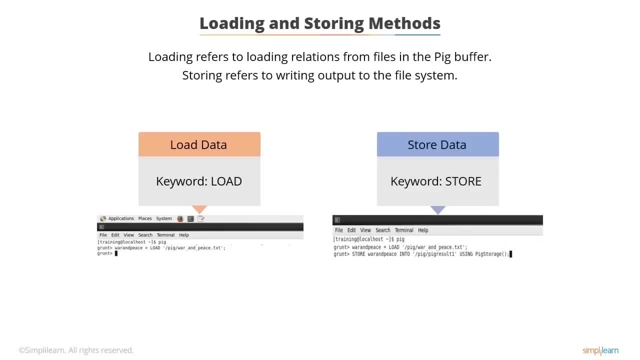 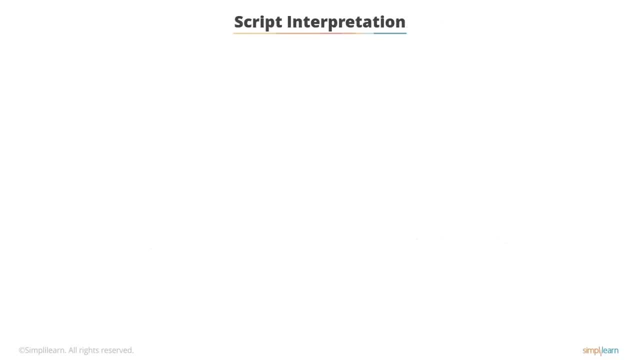 followed by the name of the variable whose data is to be stored, along with the location of storage. You can use the keyword dump to display the output on the screen. PIG processes PIG- Latin statements in the following manner: First, PIG validates the syntax and the semantics of all statements.